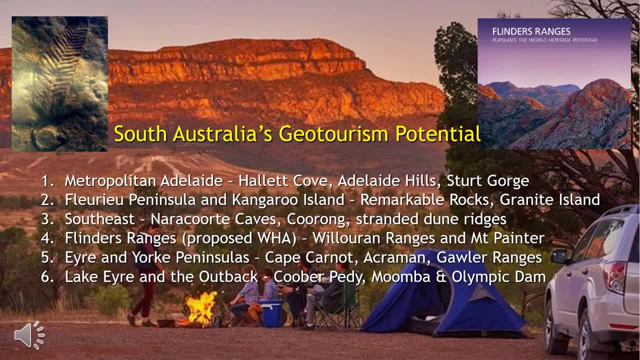 technologies and geotourism interpretation for about 30 years, So I have a very close connection with the very many spectacular geosites and georegions that we find in South Australia. For me, geotourism is all about helping the general public to. 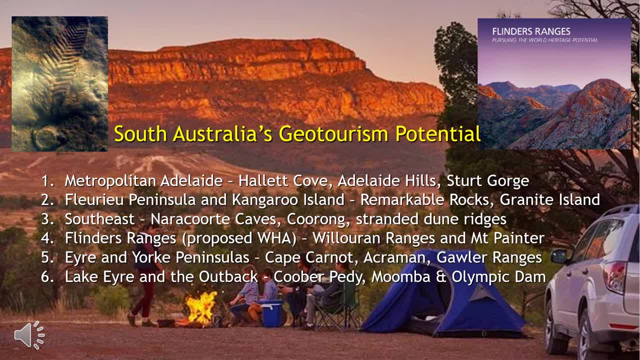 get interested in and involved in Australia's, and in particular South Australia's, amazing geological features, Also about the stories those features tell and the underlying beauty of the rocks, landforms and landscapes. This is best done by showing tourists spectacular examples of geological features. 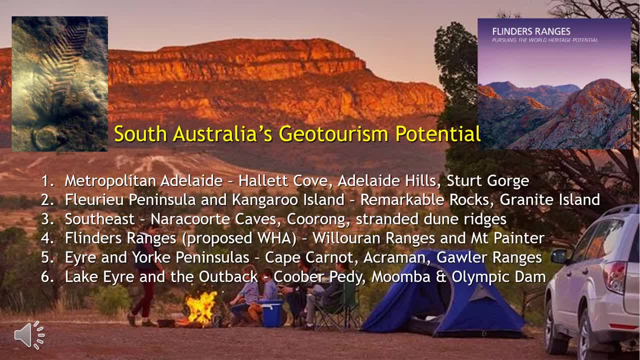 For example, geosites like geoheritage sites, and then explaining to them by geointerpretations what incredible stories the rocks can reveal. Serial examples of such geosites can be linked together as geotrails and whole geographic areas such as conservation or nature reserves. 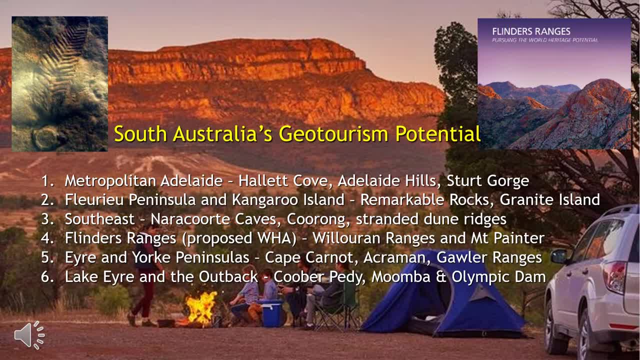 and national parks or geoparks can be used to provide a wonderful and useful geotourism experience. This current project stems from the research and development of the National Geological Survey of South Australia. It stems from my interest over the last five years as a research. 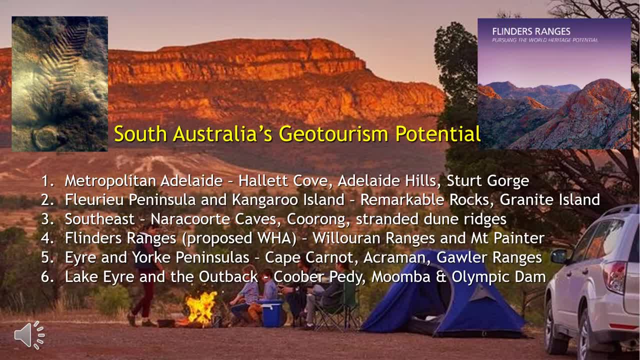 associate with Nature Foundation South Australia in conjunction with UniSA's Project Live, but also with the Geological Society of Australia in their field guides and geotourism subcommittees, and also the Geological Survey of South Australia in regard to their discovery trails. 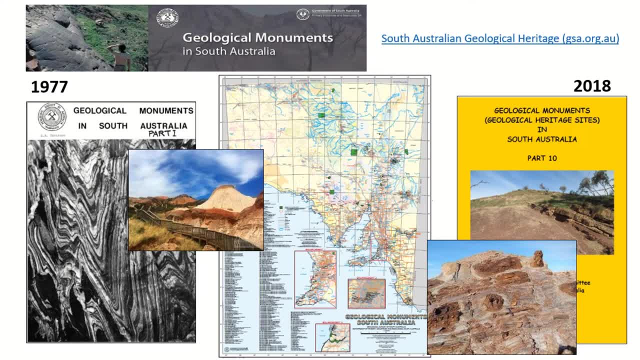 South Australia's geological monuments or geoheritage sites provide a stunning reference to potential geotourism locations or geosites and regions. These were started more than 40 years ago by my colleague, Maud McBriar from Adelaide University and the South Australian 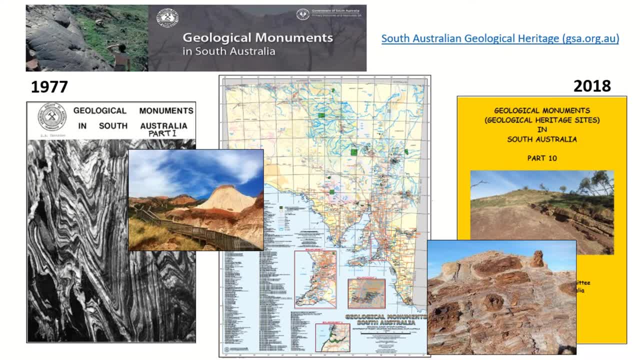 Field Geology Club. We have documented a wealth of spectacular geosites which have been carefully described and displayed in 10 volumes of the Geological Society's Geological Monuments, and there are now almost 500 sites located in all of the major geo-regions of South Australia. 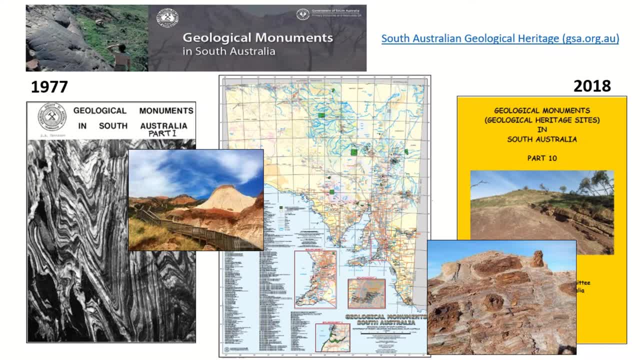 including the South Australian Geological Society, the National Geological Survey of South Australia and the National Geological Survey of South Australia. The National Geological Survey of South Australia is the largest geological site in South Australia and found on the GSA website. All are available as printed volumes, on CD and on the World. 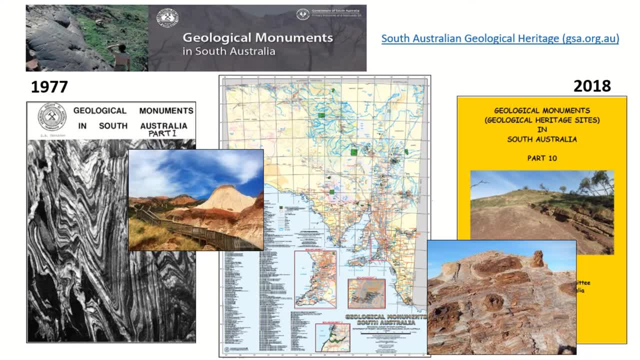 Wide Web through the Geological Survey's SARIG website and on the GSA website. By the way, the first monument listed was at Hallock Cove back in 1977 in Metropolitan Adelaide and the very last was Bubble Rocks Gully, only published a few months ago. 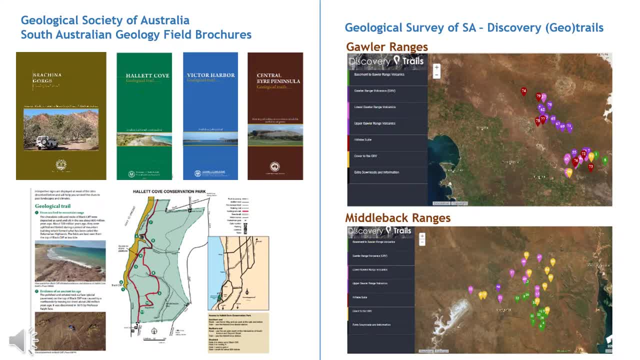 As you can see in this slide, in South Australia we already have a variety of geotourism sites, including the National Geological Survey of South Australia and the National Geological Survey of South Australia. The South Australian branch of the GSA has published 12 paper field guides, shown here. 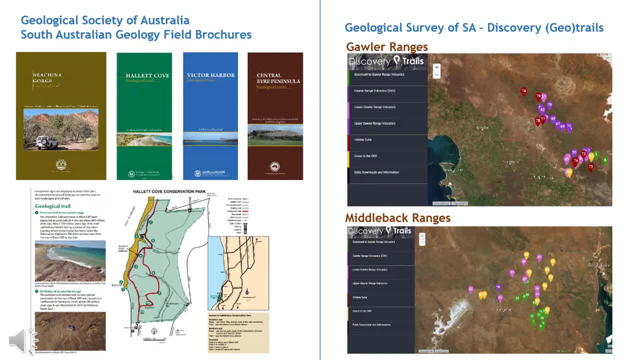 from Bratchen and Gorge, Hallock Cove, Victor Harbour and there are many others, from Coorong, Robe, Lower River, Murray to Selleck's Hill, Streaky Bay and even the building stones of the North Terrace. These are produced by people like John Cann and Barry Cooper, and 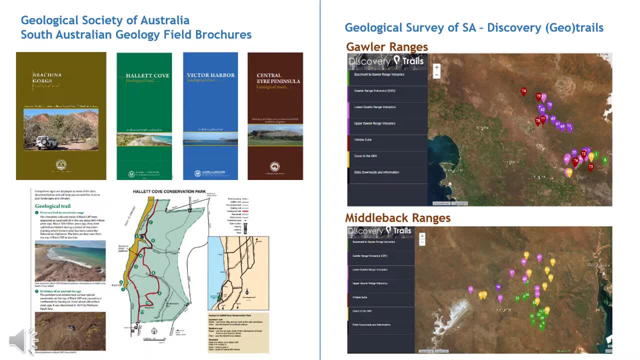 others, and there's a new one just about to be published, a wonderful one of Sturt Gorge. These guides have very simple maps and trails, some stunning images and relatively simple geo-interpretation. They tell stories like those of global climate change from the Hallock. 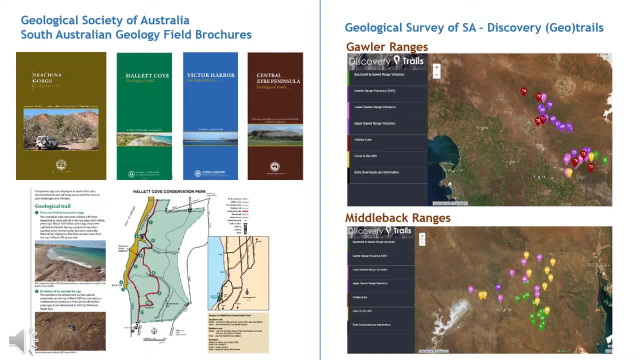 Cove, Permian glaciation and the earliest Ediacara fauna, from the Bratchen and Gorge Trail to the ancient Delamarien mountain ranges and the granites of Victor Harbour. There are no digital projects yet, but all are available online for printing and might. 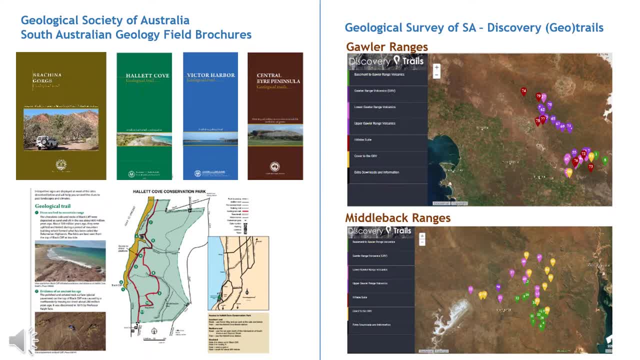 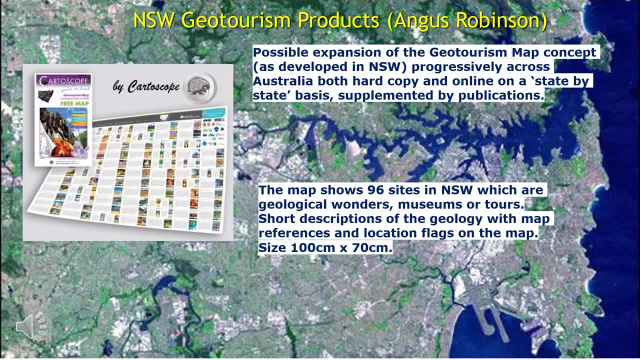 be upgraded to mobile app products in future. Likewise, as you see on the right, the South Australian Geological Survey has produced Google Earth-style discovery trails, descriptions of geo-trails and rocks from the Gawler and Middleback Ranges. This slide shows there are new geotourism materials involving my co-authors. Here's: 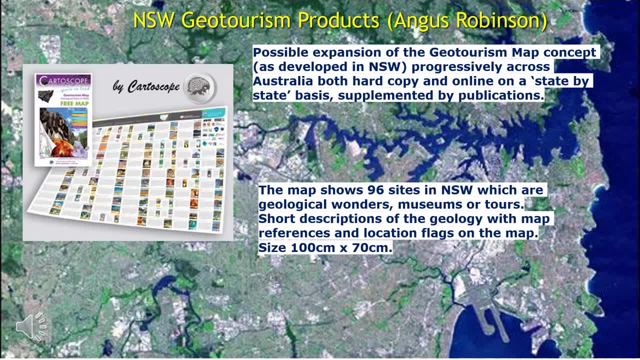 an example from New South Wales that Angus Robinson has been championing. It's the Geotourism Map Project. It's a large-scale free map and a geotourism guide with lots of geosites, locations around New South Wales, and it could be expanded to other states and maybe made 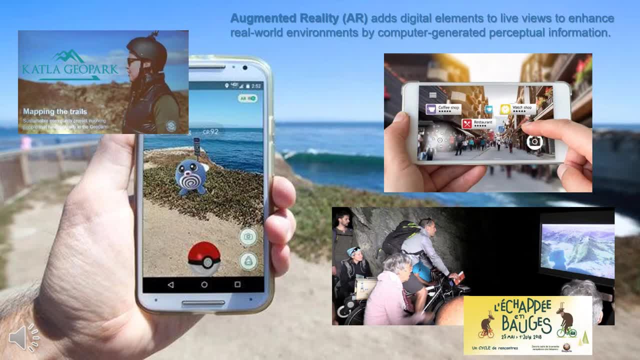 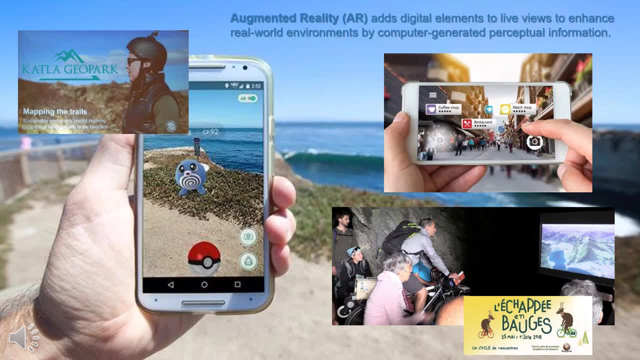 drone some software. Augmented reality can add a lot of stimulating interest to the users and the visitor experience, like the Pokemon Go app here and things like geocaching. I've seen lots of examples of this in UNESCO global geoparks around the world, like the Kattler Geopark in. 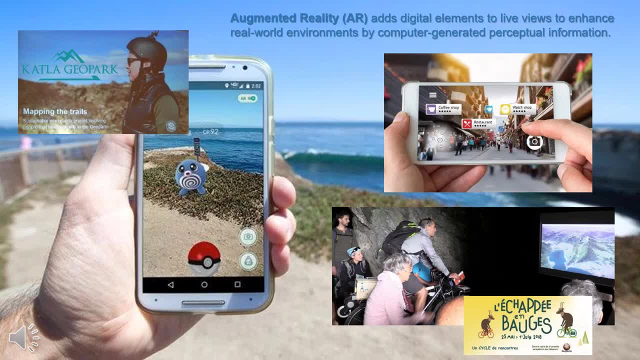 Iceland, on the top left, where GoPro helmet cameras are given to visitors on geotrails to enhance their experiences, and the Beauges Geopark in France, on the bottom right, where bicycle geotours use the energy from the bikes to drive visual geointerpretations. 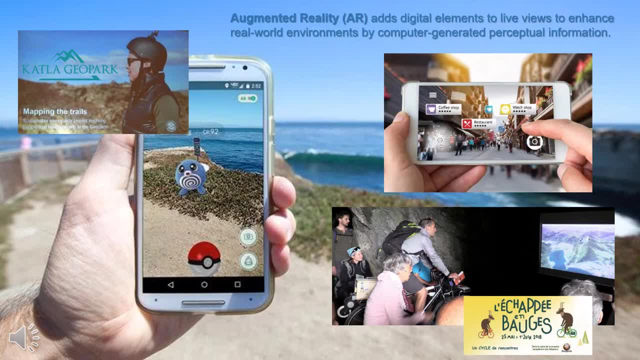 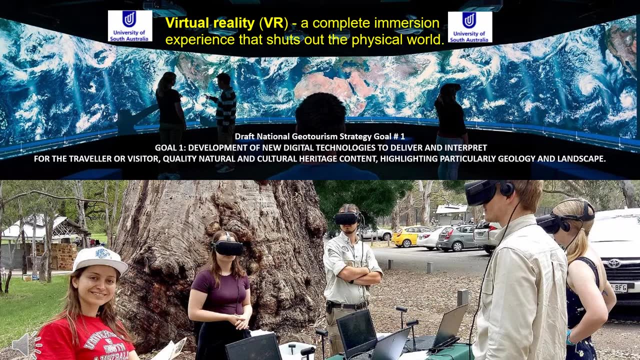 presented within magnificent limestone caves en route. So at the University of South Australia, with Project Live led by Tom Raimondo, who you've just heard from, complete virtual experiences are being developed in the new Mawson Lakes. Virtual Reality Lab And virtual field trips for students and tourists are being used to create virtual worlds. 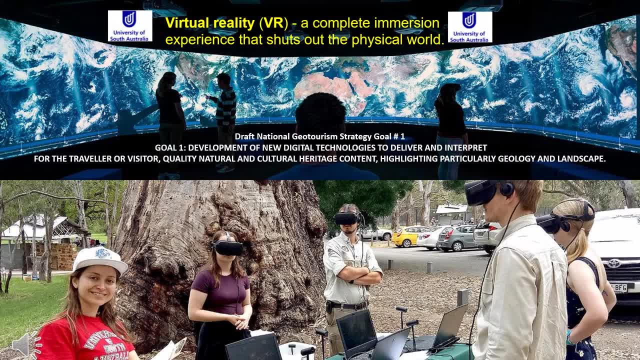 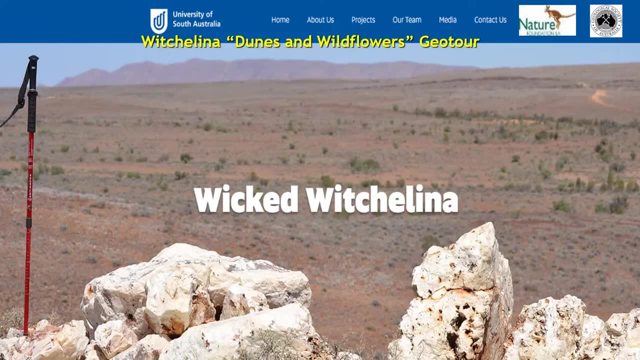 for ecotourism and geotourism and I've been very fortunate to be part of that project and to develop a couple of pilot virtual reality outback tours on the Nature Foundation Reserve where I've been developing geotrail products which we'll see in a short while. This slide shows the stunning 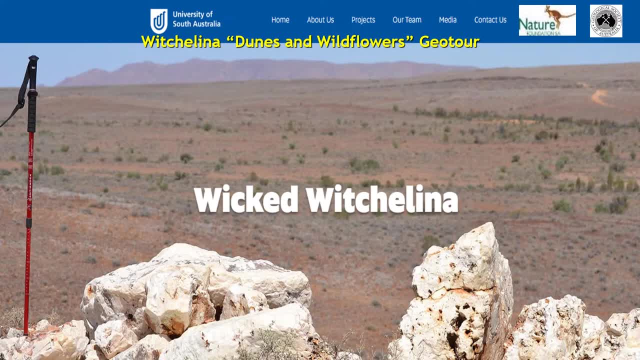 landscape of Nature Foundation's Wichalina Nature Reserve in the Wallaran Ranges, about 600 kilometres north of Adelaide, which is currently being rewilded by the Nature Foundation of South Australia. In the background is Termination Hill, flanked by the very major 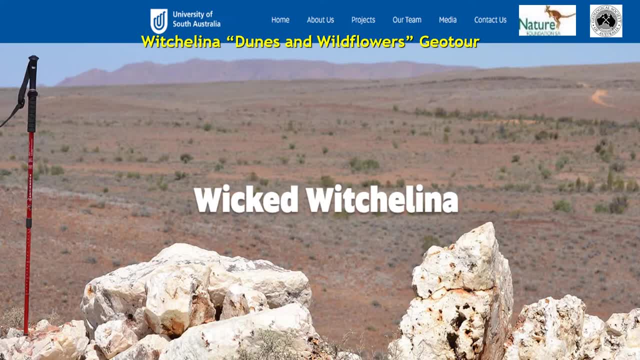 North East Fault Scarp and shows the southern limit of the 100 kilometre long Dunes and Wildflower four-wheel drive geotrails, one of many geotrails we've produced As part of the Flinders Ranges ancient Adelaide Rift Superbasin. it's got fantastic sedimentary rocks, brilliant and enormous. Delamerian. 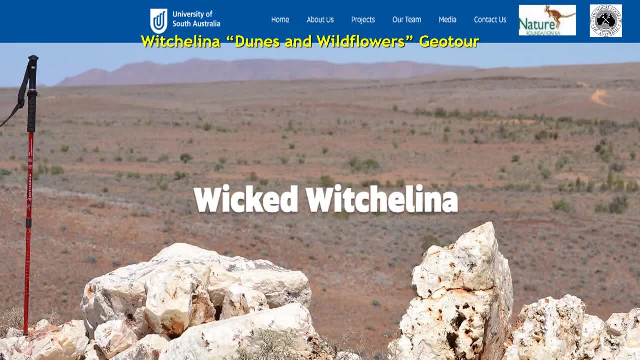 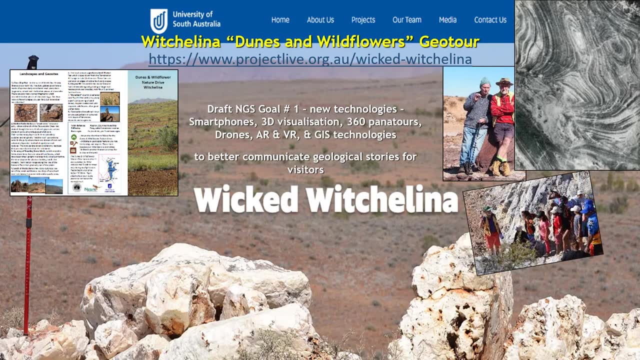 Fault. This geotour, with about 10 geosites, including bubble rocks, is described on a simple A4 brochure. Tourists who visit include Aboriginal school students, geological experts- there's Vic Gostin with me- and many other tourist groups. The drives show the geosites, but the area is most spectacular. 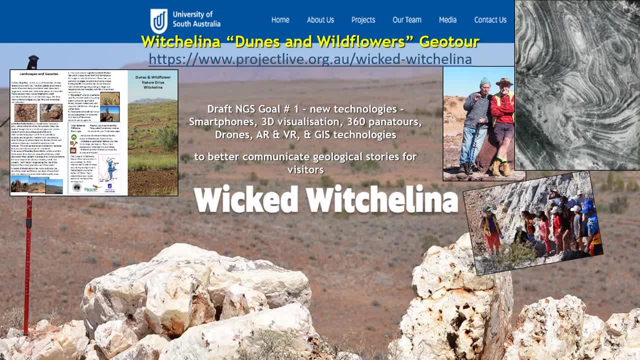 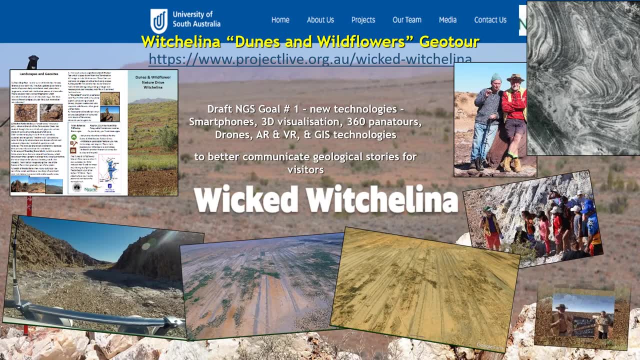 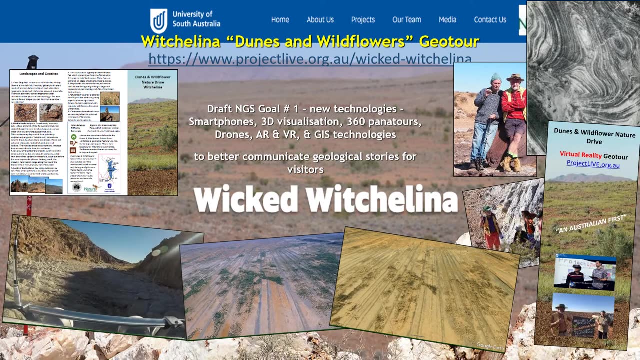 when it's seen from above, which was first recognised by Reg Sprigg when he mapped it in the 1940s And you can see from the aerial photograph image on the right. As you can see, even four-wheel driving is extreme on the very rough tracks. this one, 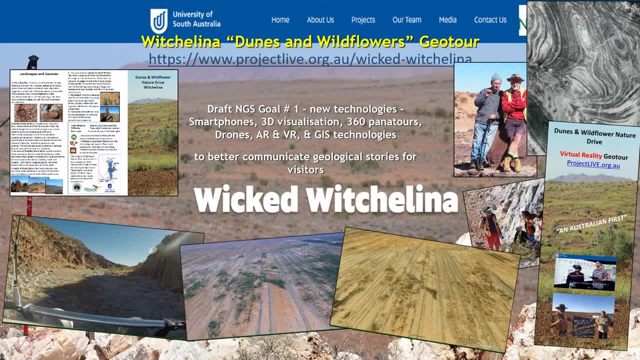 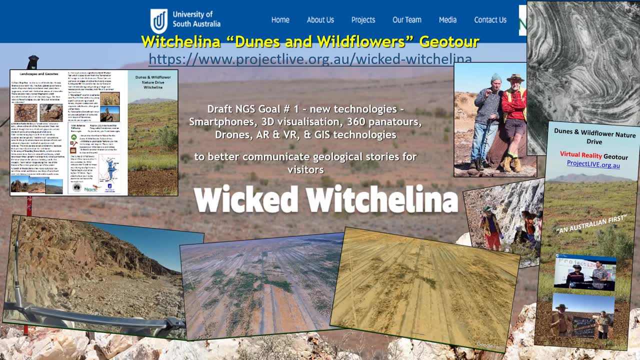 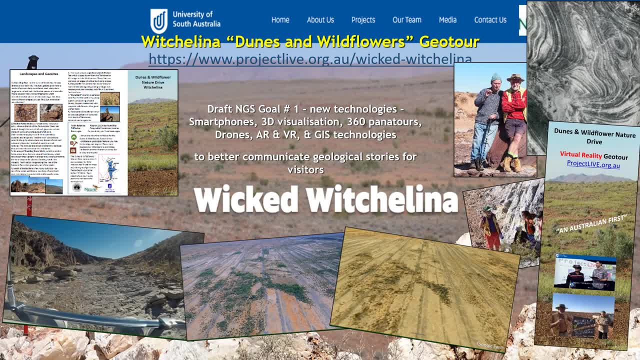 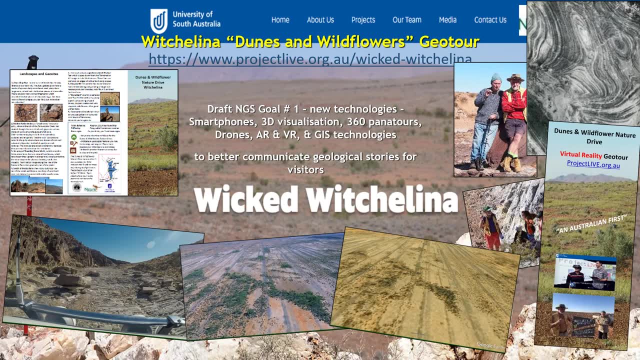 the Scalodaly Dolomite cyclothemes and the Scalodaly Dolomite planes On the right you can also see that I've been able to simulate that, that sort of flight by Google Earth Tours, and of course you can add music to that as well. 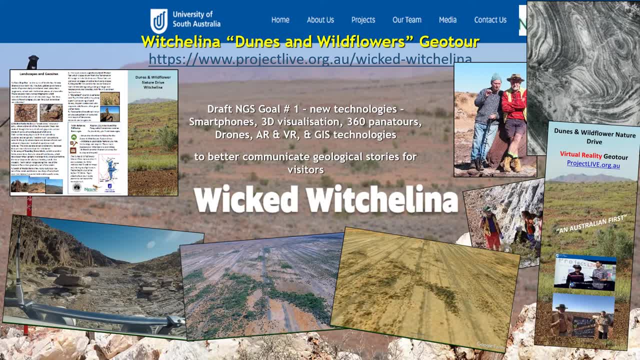 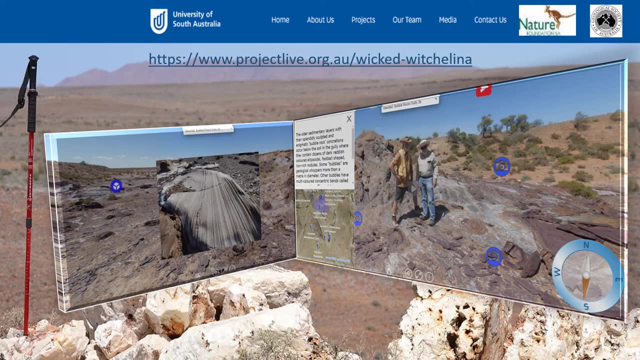 And now we've developed a virtual reality experience for marketing, promotion, accessibility, including other images and information on maps, And I'll show you this next. Unfortunately, I can't show you the virtual reality site, but here are a couple of pictures from the virtual reality immersive experience. 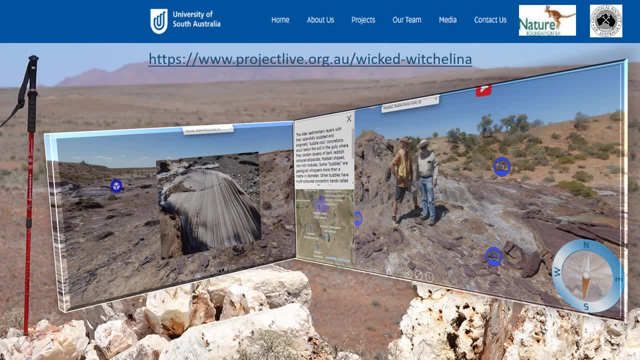 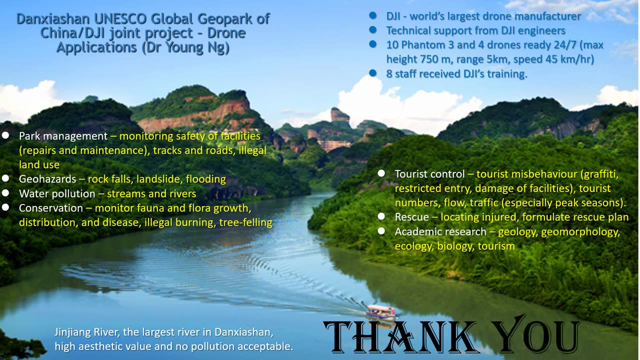 This is a 360 degree panoramic tour and we have one for each of the sites. They've got embedded video recordings and drone and GoPro video and Google Earth locations and lots more, So have a look at them for yourselves. And so back to where I started, at Dangshashan Global Geopark. 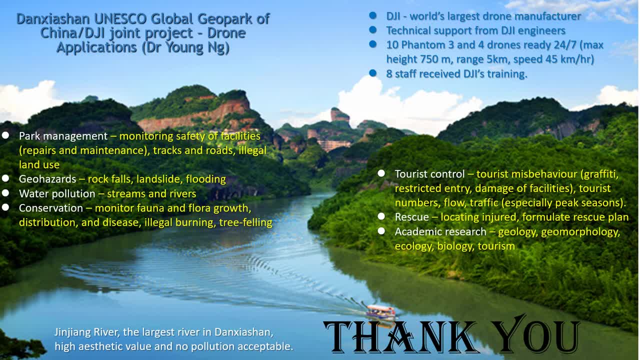 which has 250,000 visitors in 2020.. Fleets of drones being used for geotourism in the park: management, geohazards, water pollution, biodiversity conservation and lots of other things. So, finally, on behalf of my colleagues and myself,